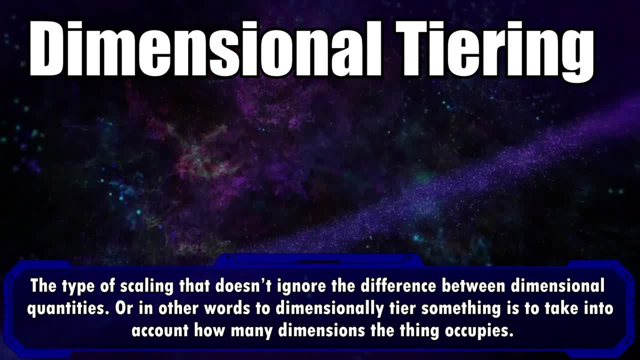 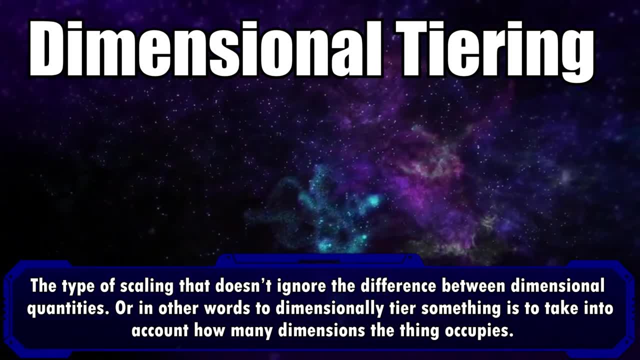 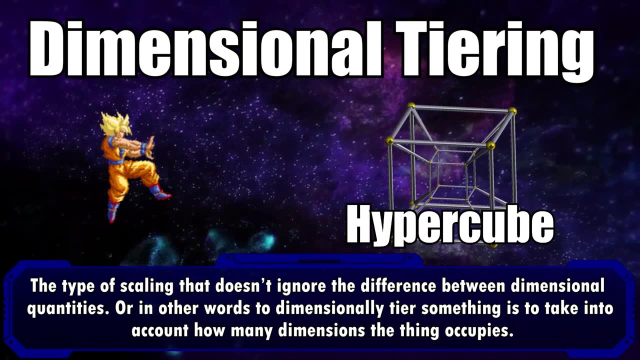 is the type of scaling that doesn't ignore the differences between dimensional quantities, Or, in other words, to dimensionally tier something is to take into account how many dimensions the thing occupies. So, for example, if a character destroys something, If a character destroys a tesseract, also known as a hypercube, using dimensional tiering. 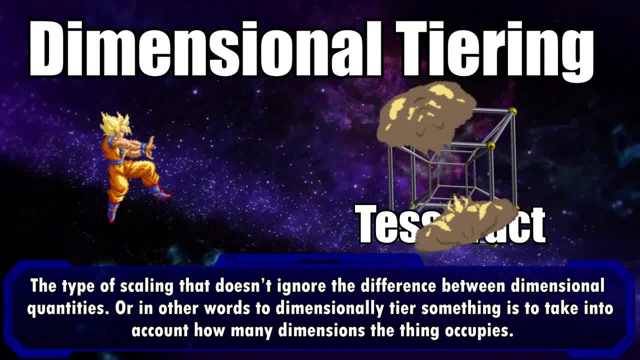 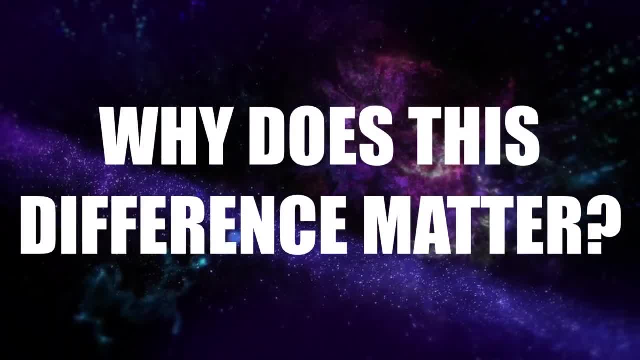 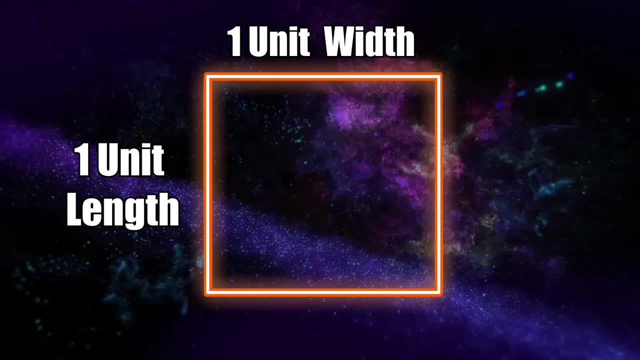 this would be a 4th dimensional feat, since tesseracts or hypercubes are defined by being 4th dimensional. So why does this difference matter? Well, let me give you an example to show you how important this difference is. Let's take a square with a length and width of 1 unit. 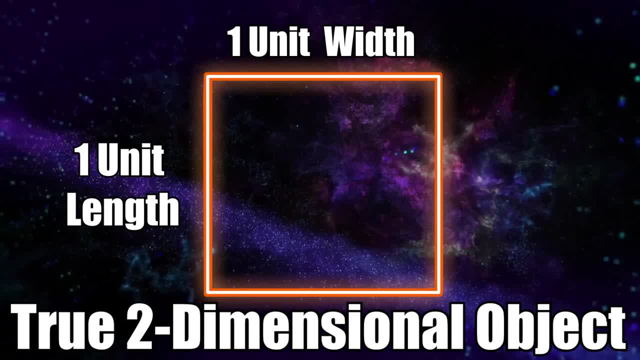 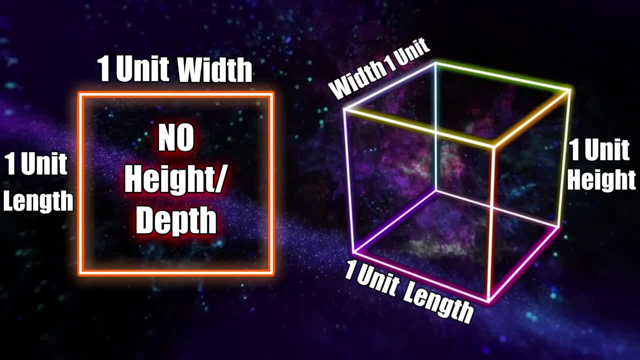 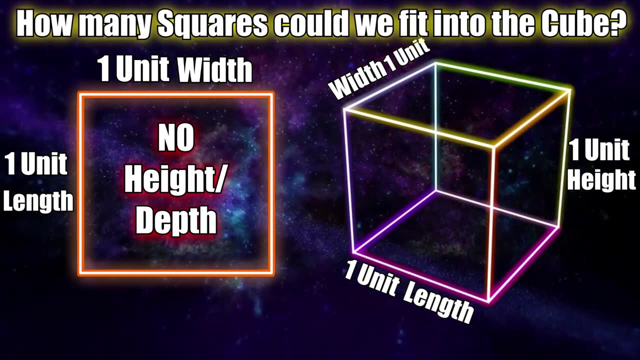 This square is a true 2 dimensional object and thus has absolutely no height at all. And if we compare it to a cube with at least one dimension, with width and height, How many squares could fit into the cube? Well, the square has no height or zero height. 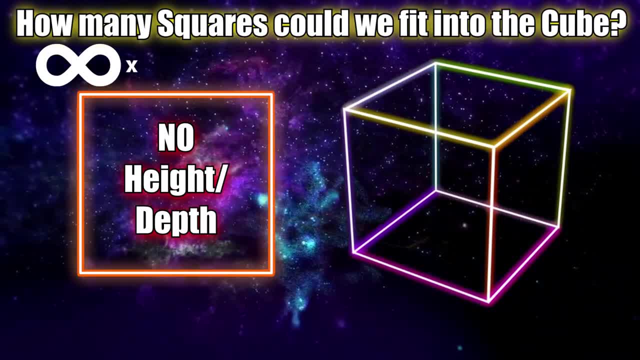 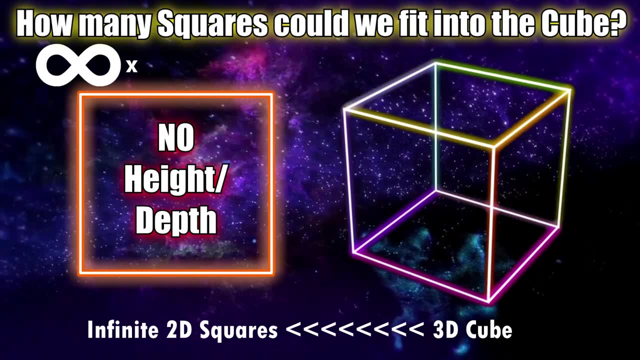 so even an infinite amount of squares stack on top of and around of each other wouldn't make a cube. So to ignore dimensionality is to ignore just how many squares the cube fits into it. This is the same trouble of how many zero's are needed to fit into each other to reach. 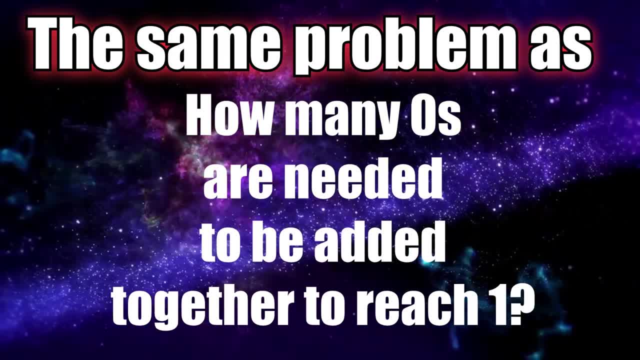 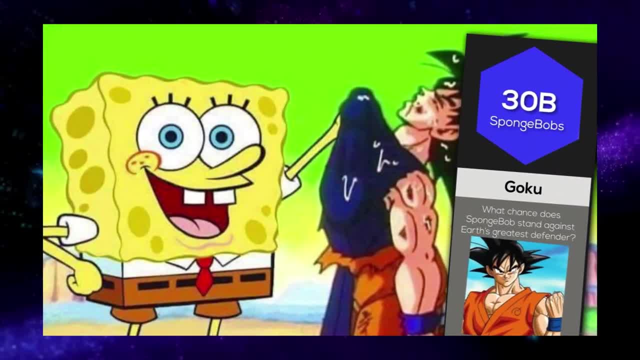 the number that leaders and minus метres of a cube are small. for the New mechanism to今年 to be a 3Da one, To go in reverse of how many squares this cube level person can destroy. we have to talk about ways to measure energy, which would be in joules A joule. 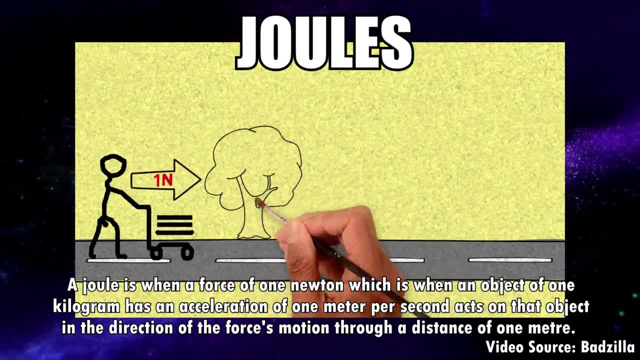 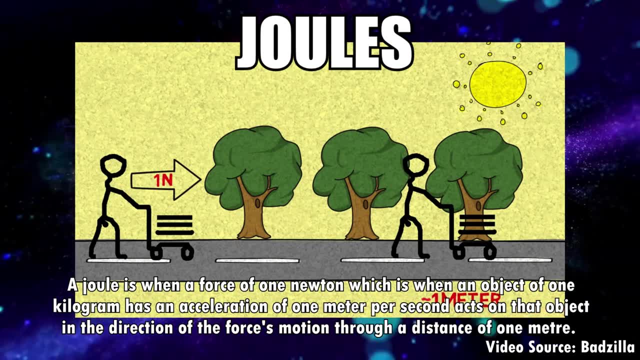 is when a force of one unit, which is when an object of one kilogram has an acceleration of one meter per second, acts on that object in the direction of the forces motion through a distance of one meter. So joules are in part defined. 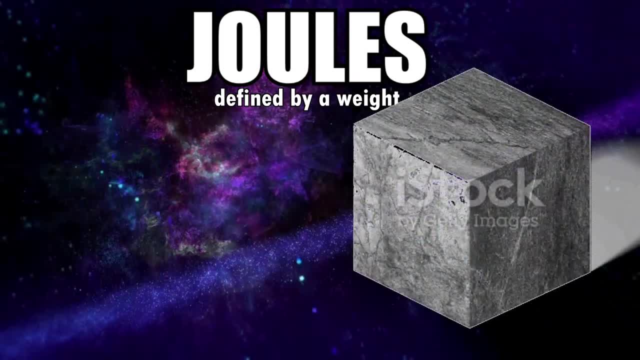 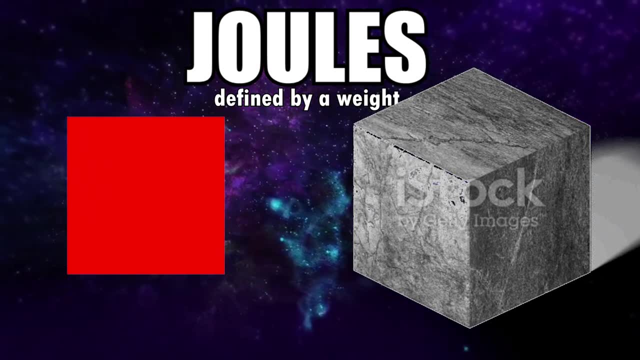 by a weight. Obviously, something like a 1 by 1 by 1 meter cube of rock has a solvable weight, but for a perfectly flat square this is less obvious. It doesn't even really make sense to apply a weight to something that is similar to the. 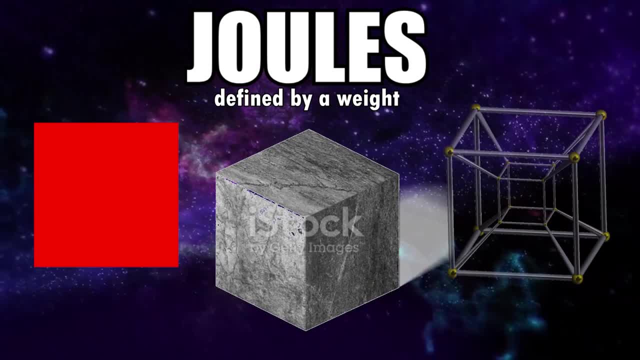 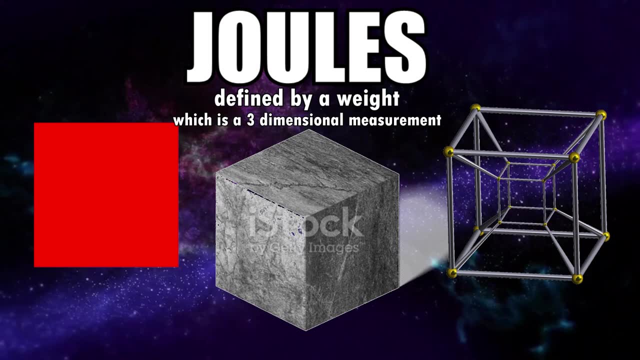 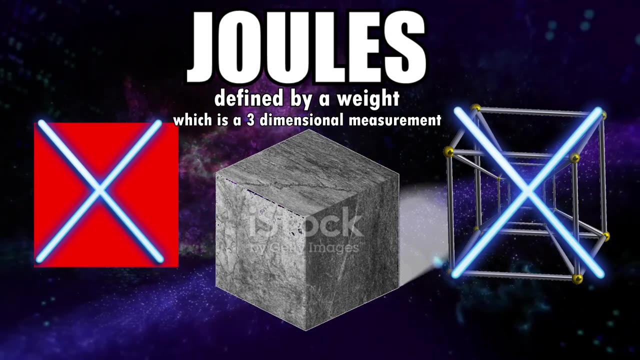 number of zeros needed to reach one. A weight like a kilogram is exclusively a three-dimensional measurement, which means that normal joule values cannot be applied to a higher or lower dimensioned object Without producing ridiculous results like beyond infinite joules, which isn't. 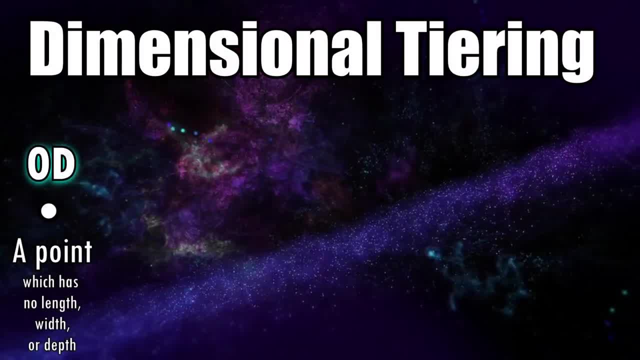 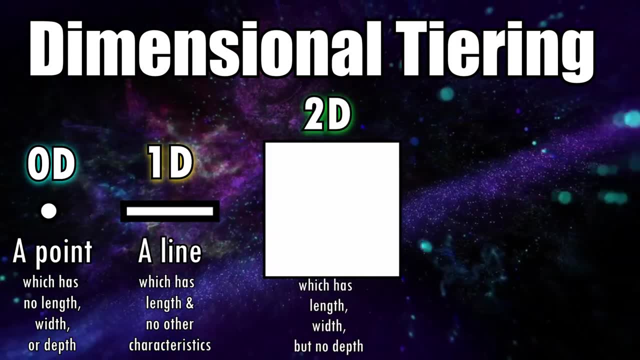 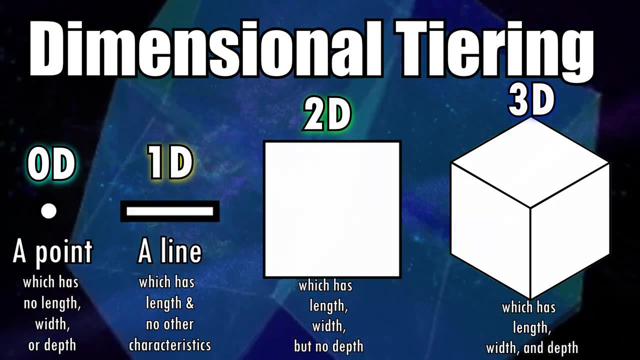 very useful. A point is a zero-dimensional object, A line is a one-dimensional object. Something like a square is 2D and something like a cube is 3D. But how do we deal with objects with more than three dimensions? And what? 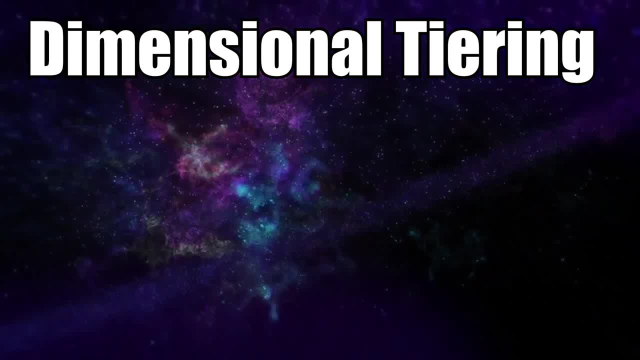 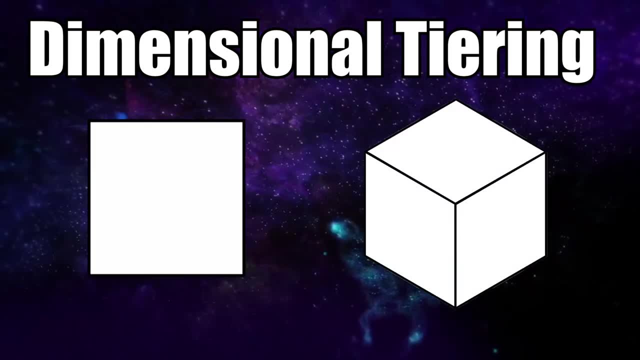 even is a fourth-dimensional object. Well, to start talking about objects with more than three dimensions, we need to know how to measure energy. So we need to look back at our good old friends the square and the cube. With how many squares can be stacked into the cube, or how many zeros are needed to reach one? 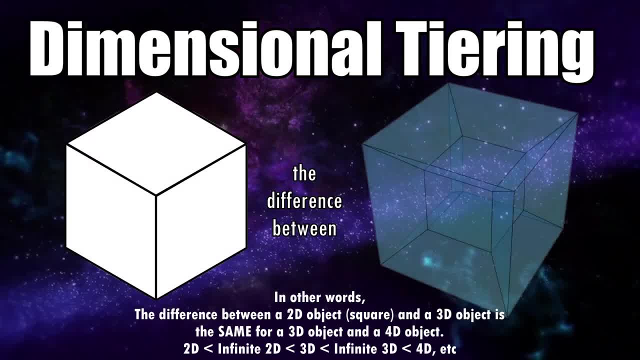 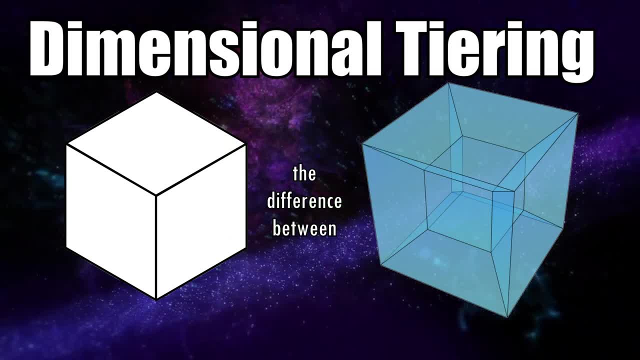 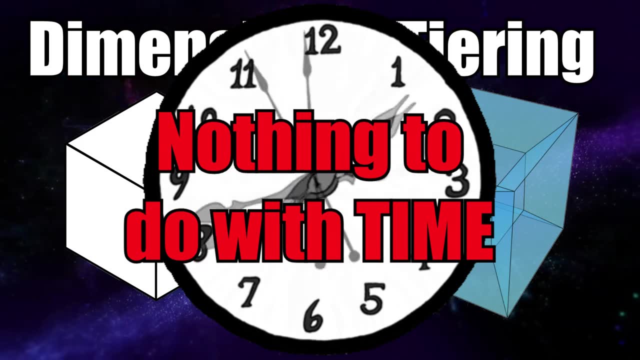 we need to understand that the difference between a cube and a hypercube or tesseract are the same. It's important to know here that this difference has nothing to do with time, which a lot of people misconstrue as the fourth dimension or something similar. 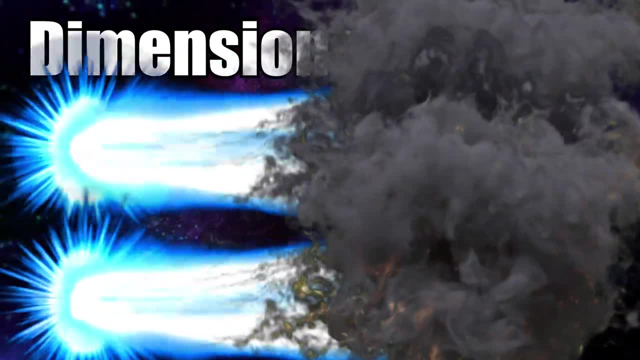 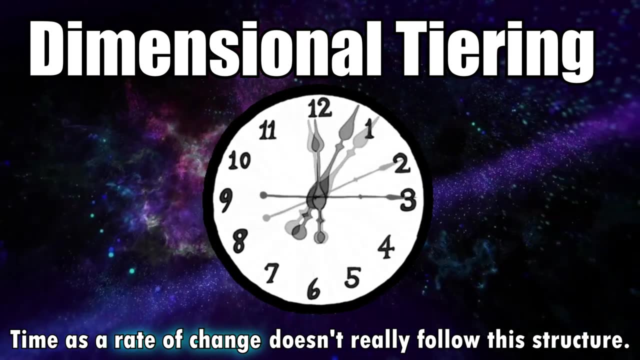 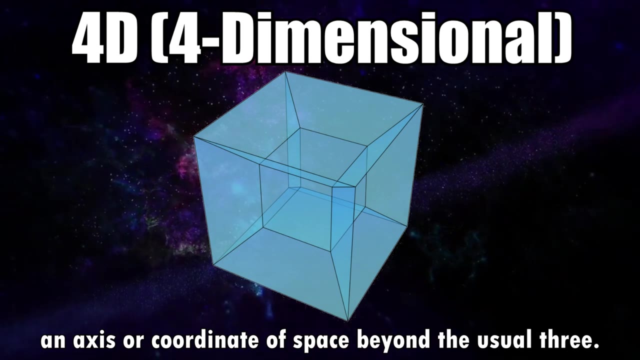 Taking time away from a cube wouldn't make it any easier to destroy, and time as a rate of change doesn't really follow this structure that we have laid out here as the next step. beyond a cube, What we mean here by 4D is an axis or coordinate of space beyond. 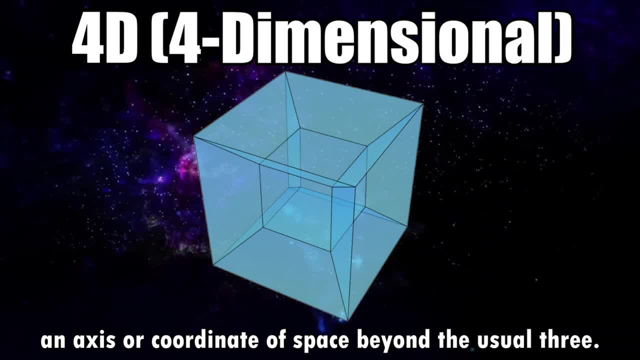 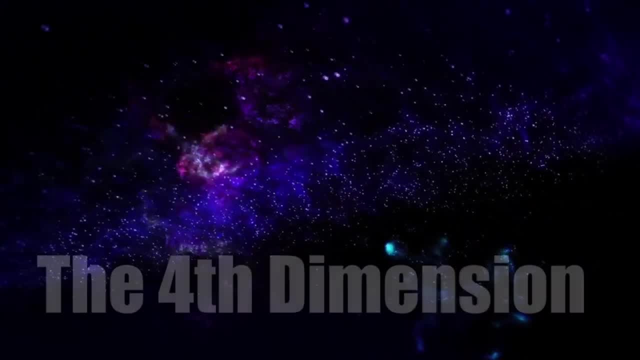 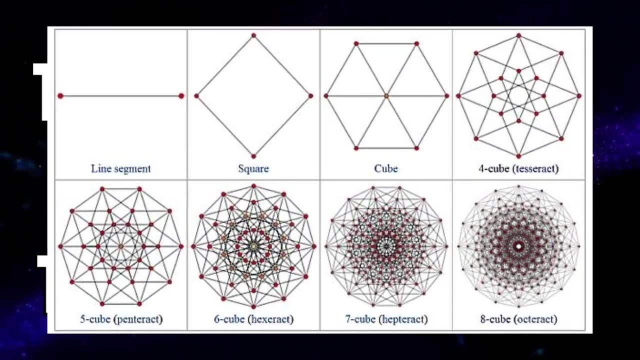 the usual three. It's hard to understand what this is like, because we don't seem to perceive dimensions beyond three. It doesn't even really make sense to say something like the fourth or the third dimension. There's nothing special about each dimension. They are all just lines at different angles, even if these angles 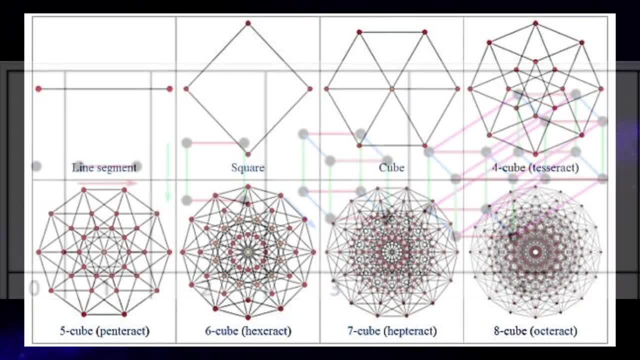 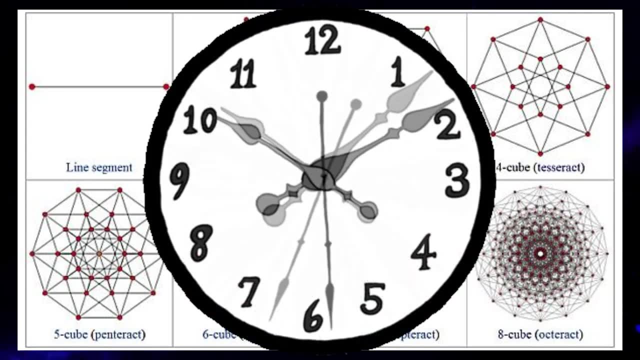 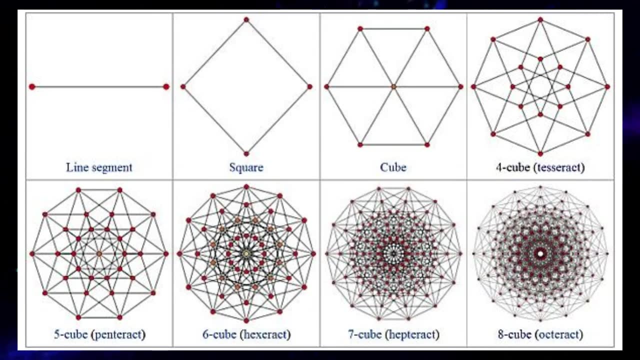 are pretty extreme. We can only really talk about an object or space having two or three or whatever number of dimensions. In this sense, it doesn't work to count time amongst these either, because it is known to be very different from any of the others, which are all identical and there also isn't really. 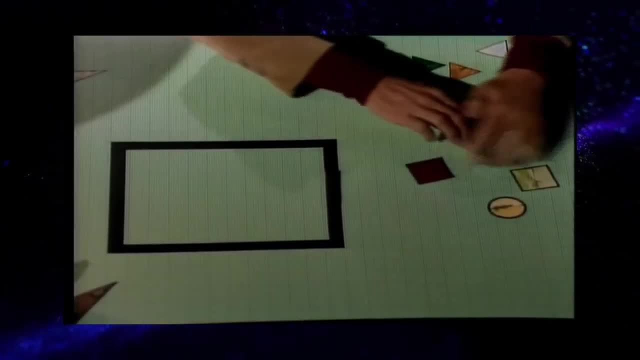 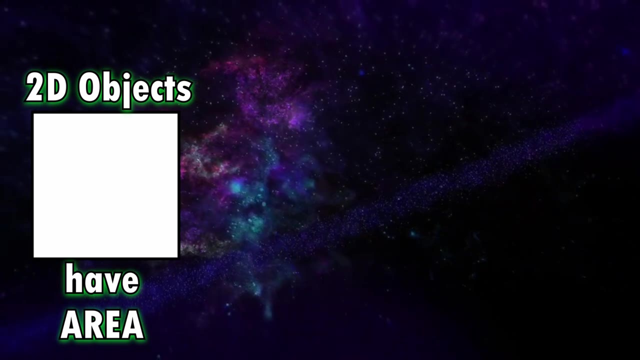 any reason to think of it as the fourth. A purely square world could have time and a rate of change. so we can describe 2D objects as having area, 3D objects as having volume and a 4D object would have something called. 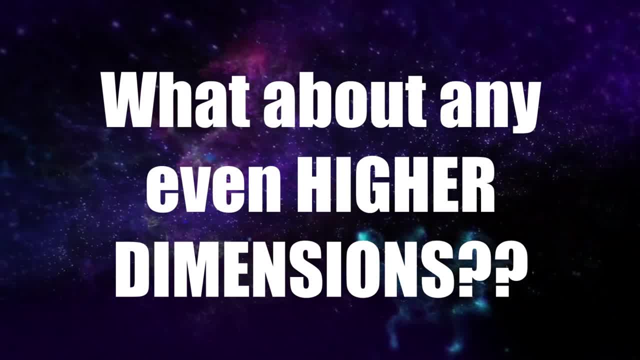 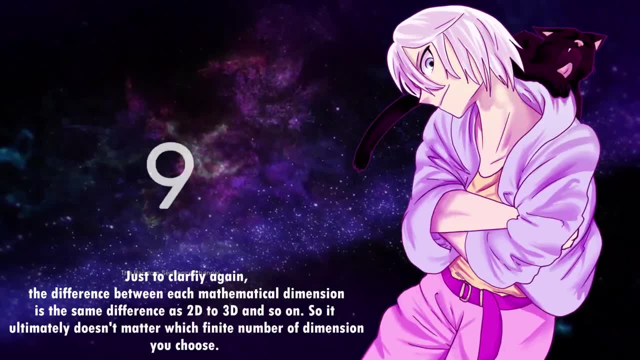 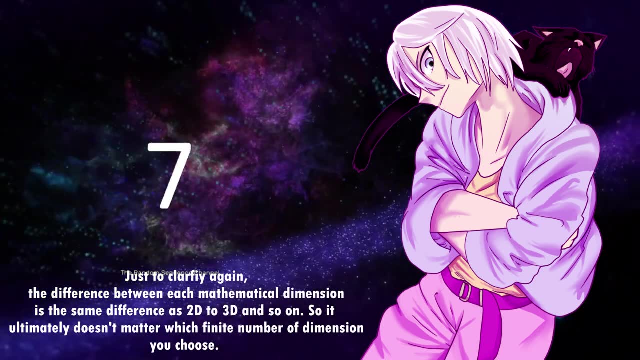 hypervolume. So what about even higher dimensions? Well, we can do this extension from a cube to a hypercube any number of times, Literally pick any number you want, and that object or space could have that many dimensions And it would be superior to each previous dimensioned object or space following the same pattern. 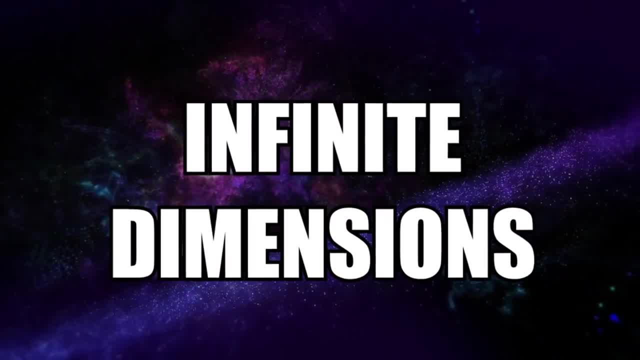 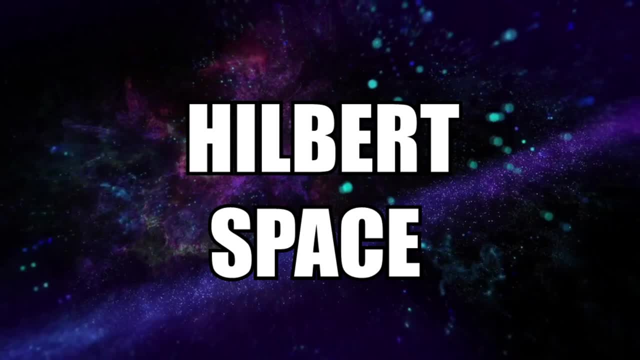 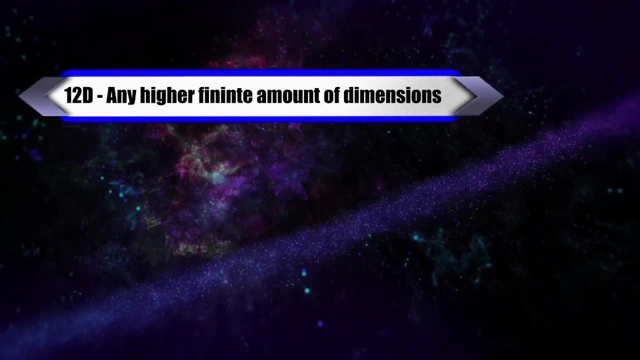 Even infinite dimensional objects or spaces are fine and real-life ways of calculating these even exist, like with something known as a Hilbert space which can account for infinite dimensions. People often refer to 12 dimensions or any other finite number higher as hyperversal. 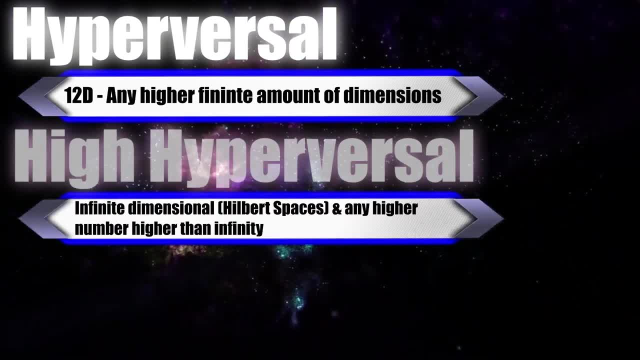 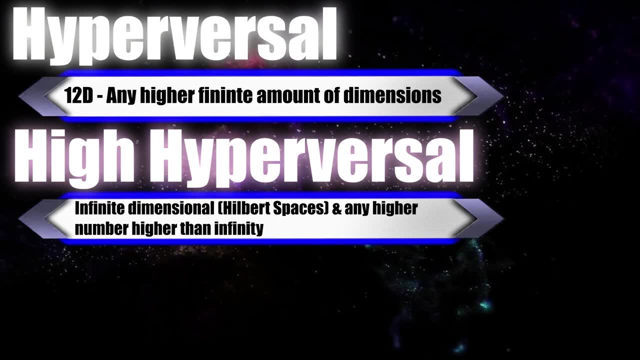 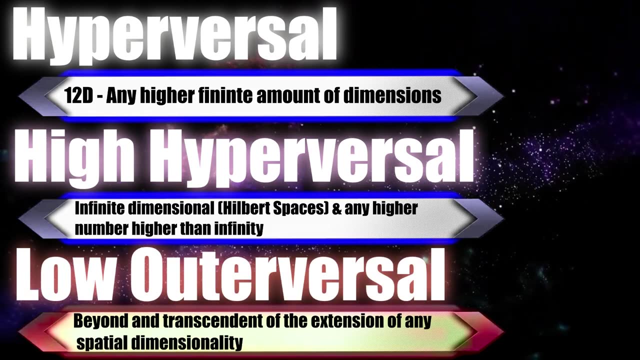 Then infinite dimensions and beyond is known as high hyperversal. We can extend this dimensional difference principle to any extent that we like. in objects or spaces that go completely beyond any extent of dimensions we call low-outerversal. Actually, the difference between low-outerversal and high-hyperversal is bigger even than the 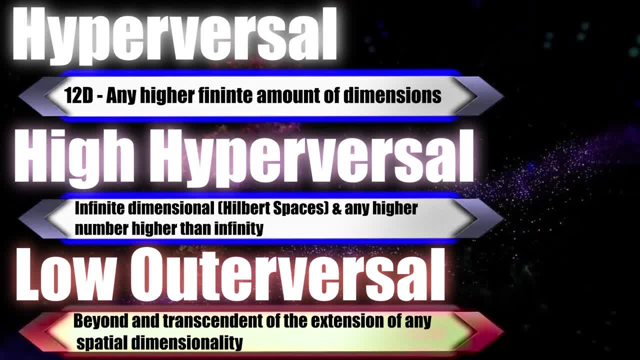 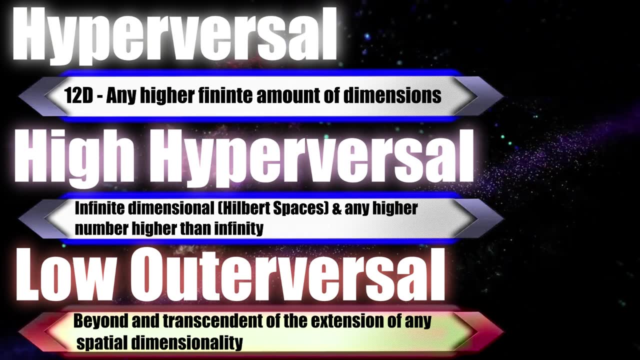 difference between a 3D object and a high-hyperversal one. to give you an idea of how impressive this is. Despite popular belief, you can't simply reach the tier of low-outerversal by simply stacking infinite dimensions on top of each other and then some as low-outerversal would. 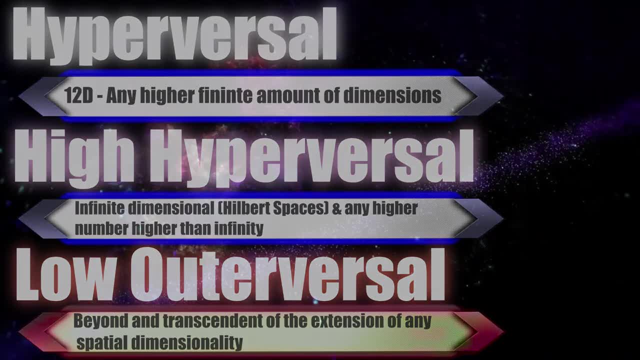 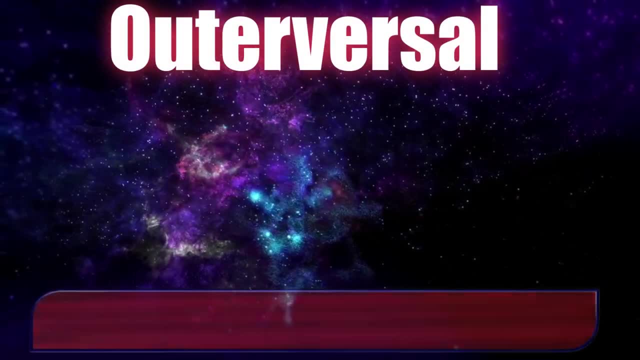 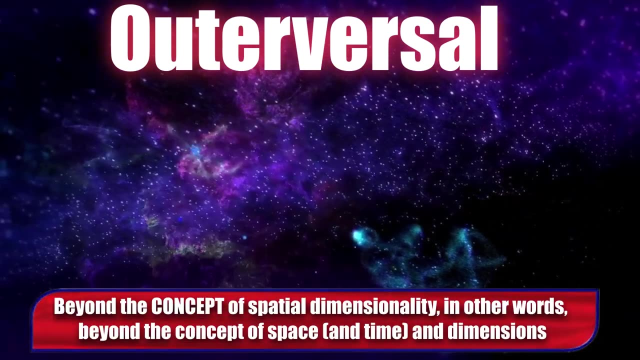 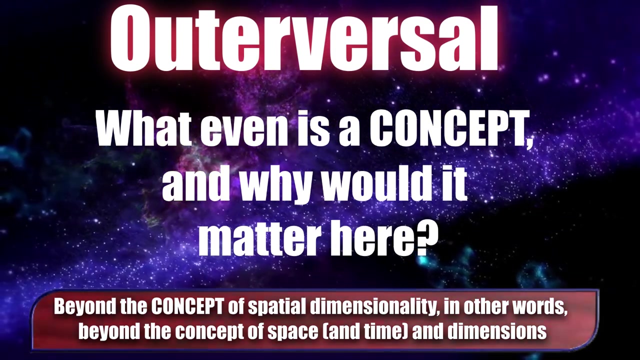 be beyond the restrictions of dimensionality in total. So that's low-outerversal. What would be the qualifications for baseline-outerversal? Well, outerversal, not low-outerversal, is being above the concept of spatial dimensionality, Which then begs the question: what even is a concept, and why would it matter here? 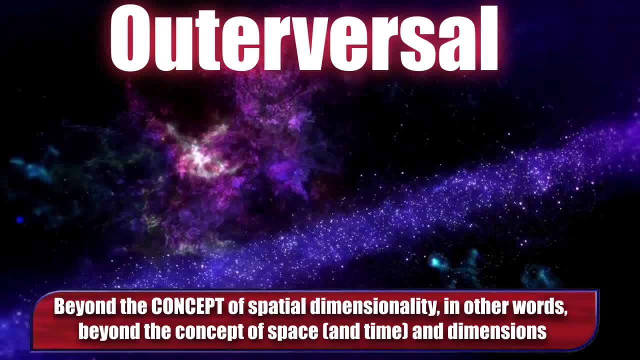 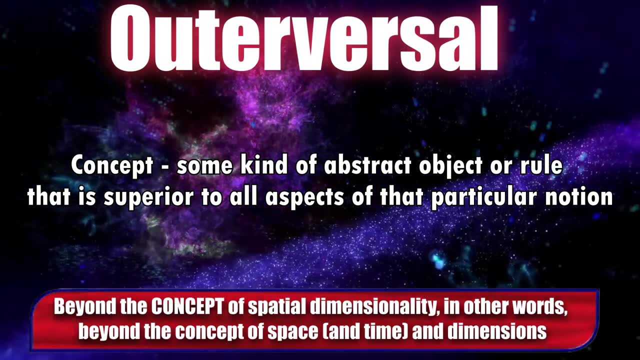 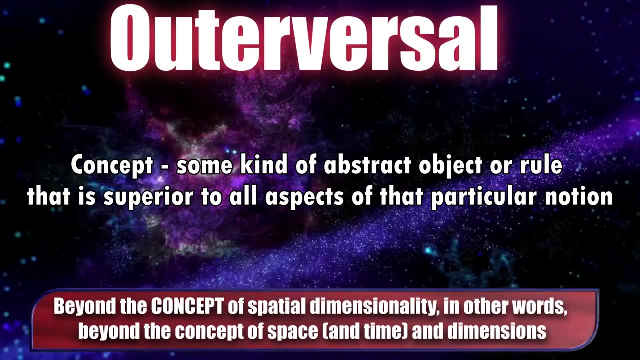 A concept can mean many, many different things, But in this case, a concept of something refers to some kind of abstract object or rule that is superior to all aspects of that particular notion and makes the thing that it's about even possible in the first place. 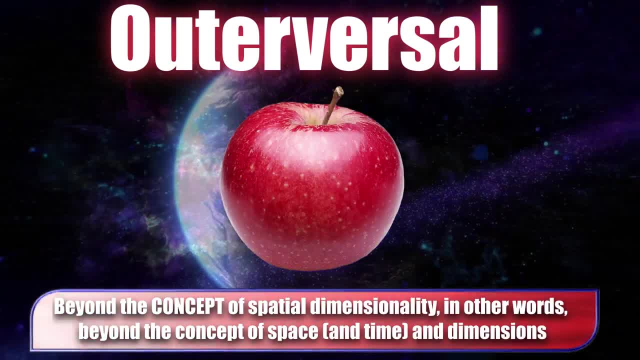 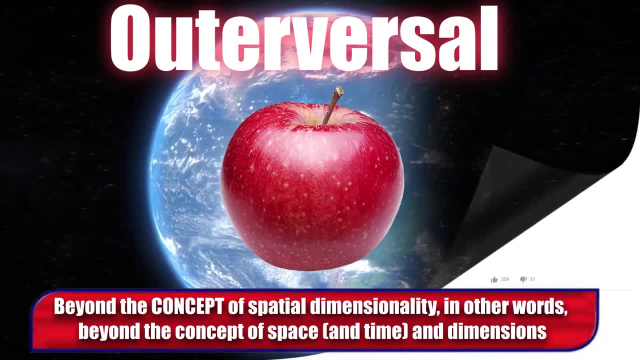 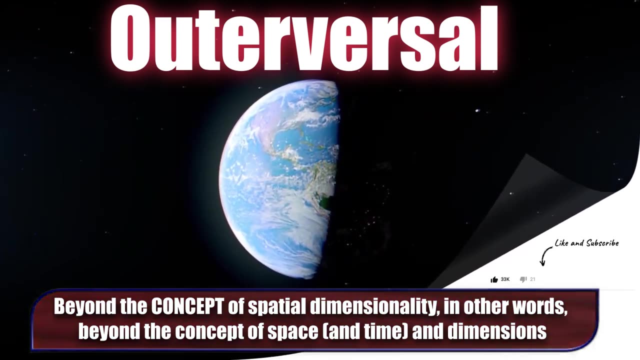 For example, the concept of an apple, in this particular meaning of the term concept, would be superior to all possible apples and would be the thing that makes those apples even possible at all. So, in this case, being beyond the concept of dimensionality is more impressive because 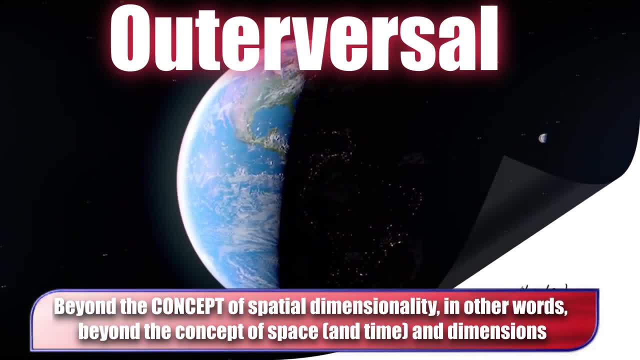 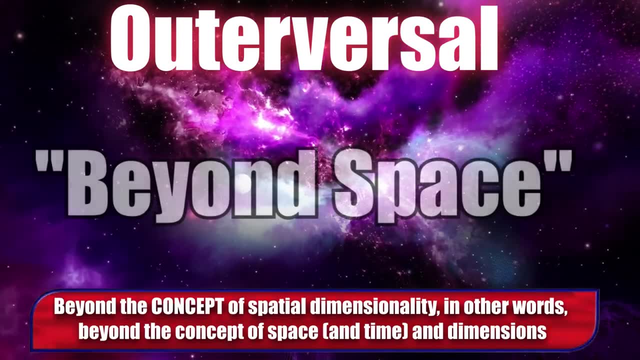 this is what makes it possible for dimensionality or space to occur in the first place. This is why this specification is important, as it doesn't equate to simply being beyond space, As, with additional context, it could easily be referring to something being beyond a 3D. 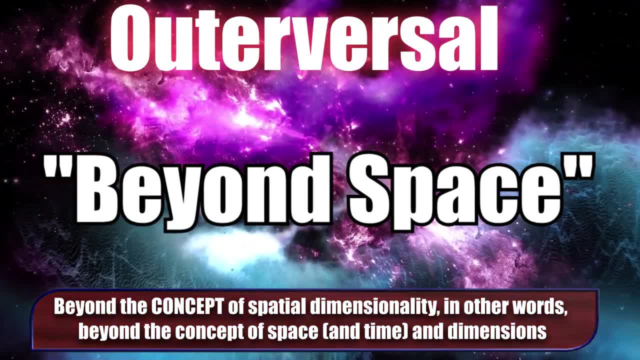 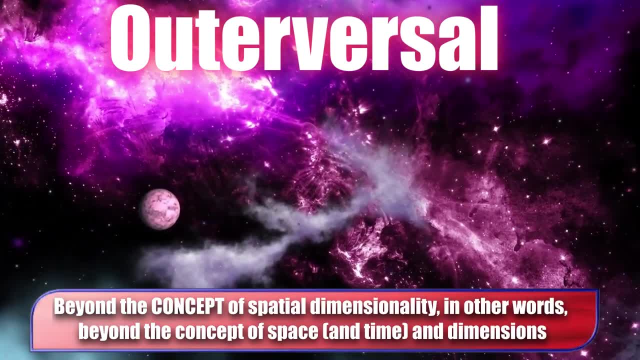 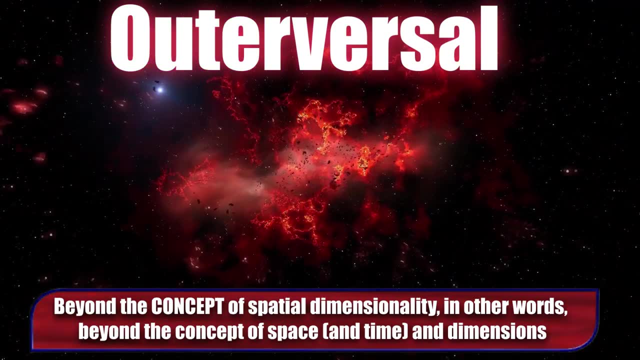 space which would make you 4D, Or being beyond 4D space which would make you 5D, etc. The point here is that something simply being beyond space is vague and lacks the predictive power to definitively mean something like being beyond the concepts of space would. 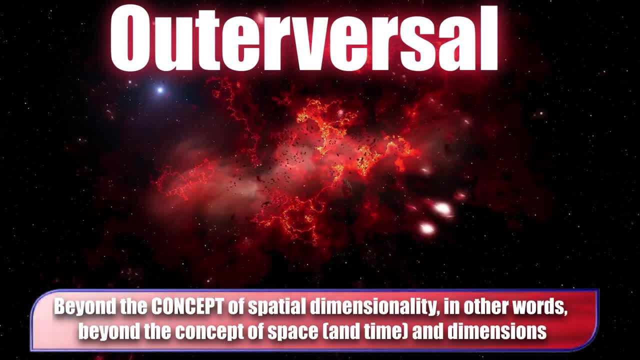 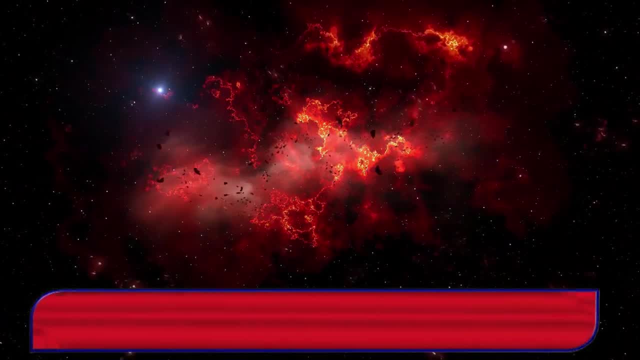 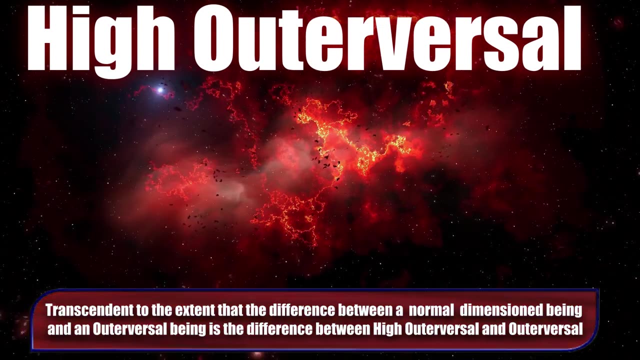 Additionally, the concept of space would also encompass all dimensionality as dimension. space is merely a type of space Which then brings us to high outerversal, which is simply being beyond an outerversal thing, to the same extent that a normal outerversal thing is beyond normal human beings. 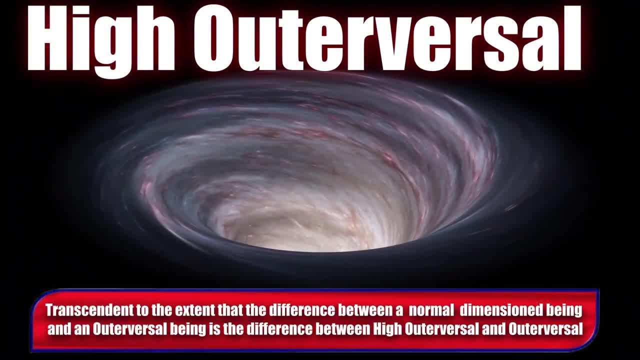 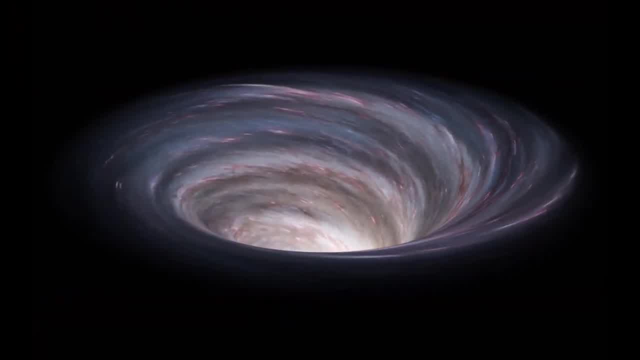 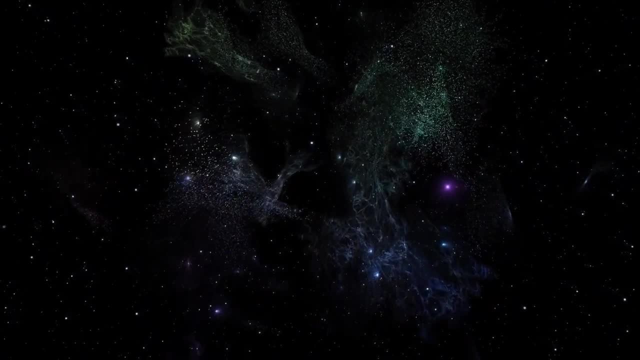 Now, hypothetically, we could invent tiers above this, but for the sake of the video, high outerversal includes everything above this. Now that we've talked about what is actually beyond dimensionality, we can now talk about things that aren't, such as transfinite amount of dimensions. 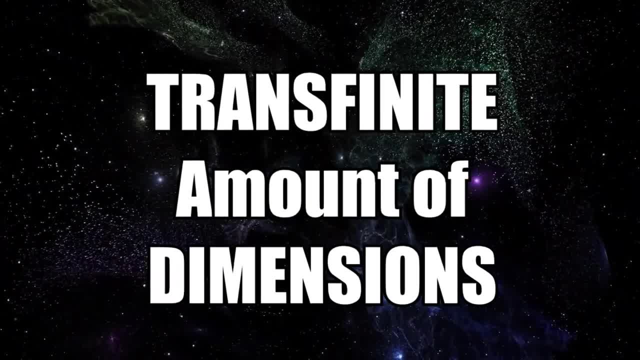 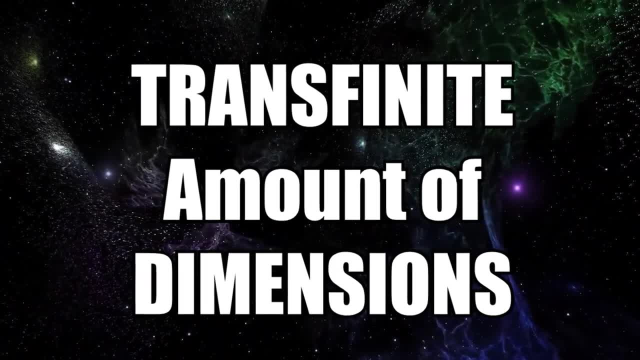 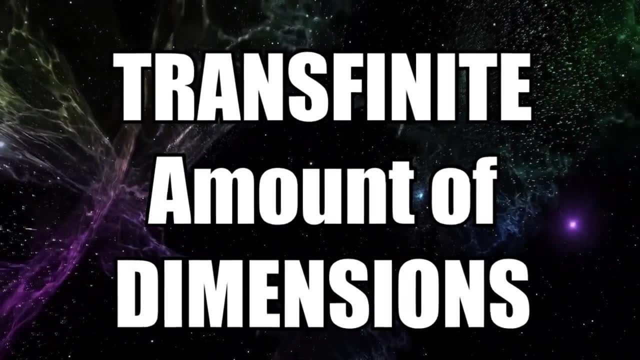 Obviously, by having a specific amount of dimensions means you are still bound by dimensionality. So hypothetically you define a tier as having aleph-null dimensions. That would be less impressive than someone who is unbound by dimensionality and also just wouldn't be what we defined as outerversal, instead of being higher into what we would. 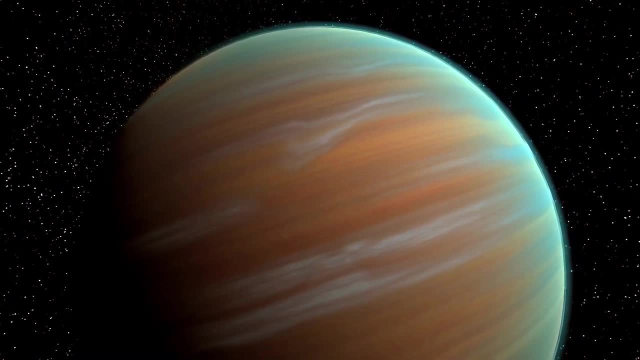 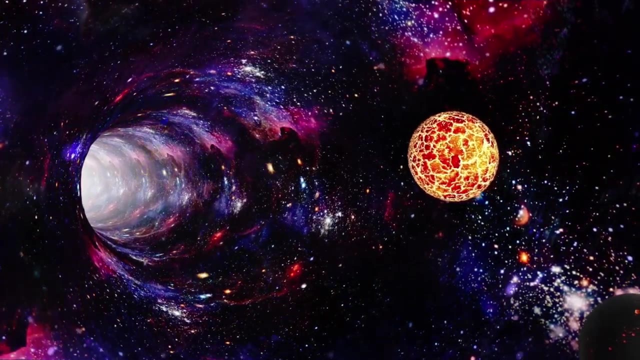 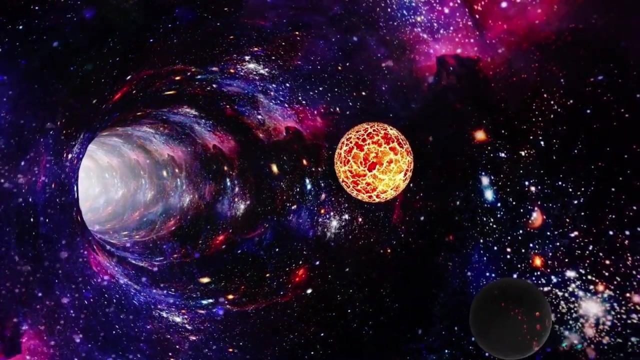 call high outerversal. I should also mention that simply having a transfinite number mentioned doesn't mean anything. In order to actually be useful, it has to relate to an amount of things, be it planets, universes, dimensions, etc. 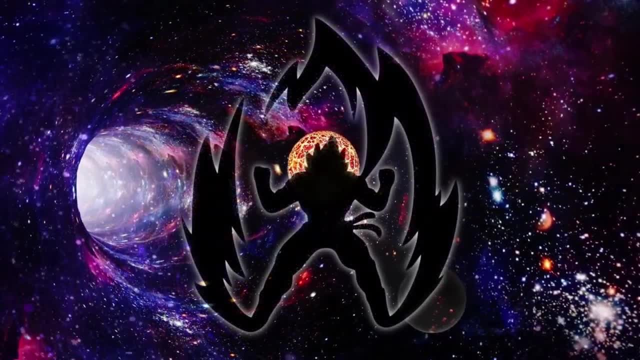 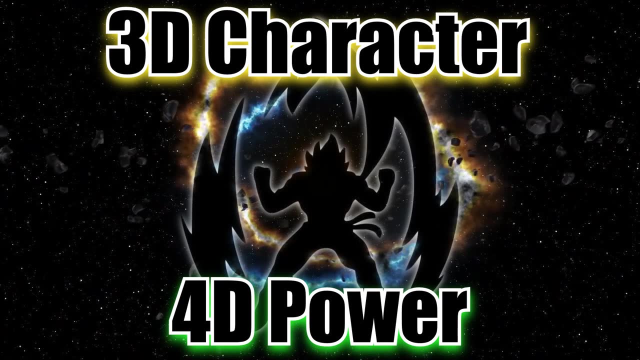 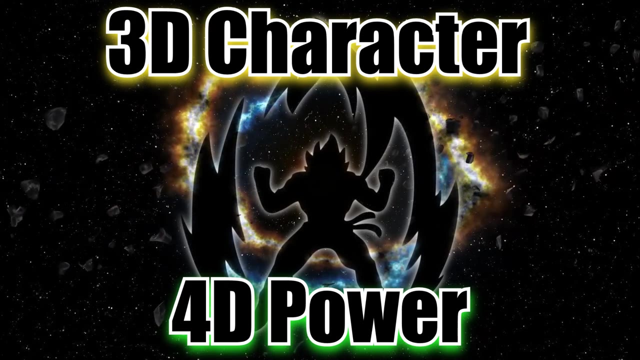 Lastly, I'd like to mention that you can have higher dimensioned or even beyond dimensioned ap without the existence of being on that level. So a character could be 3d in size while still affecting things with more than three dimensions.